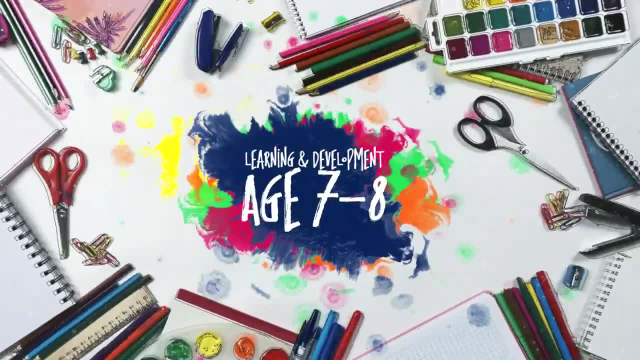 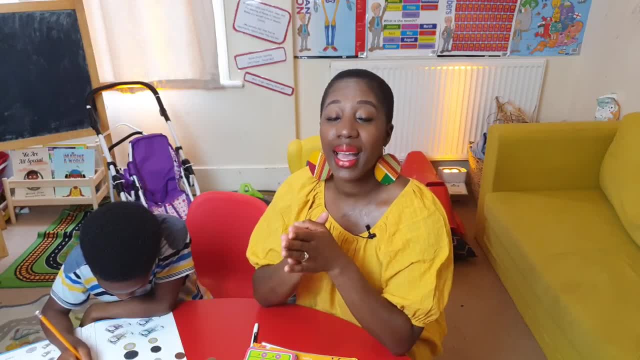 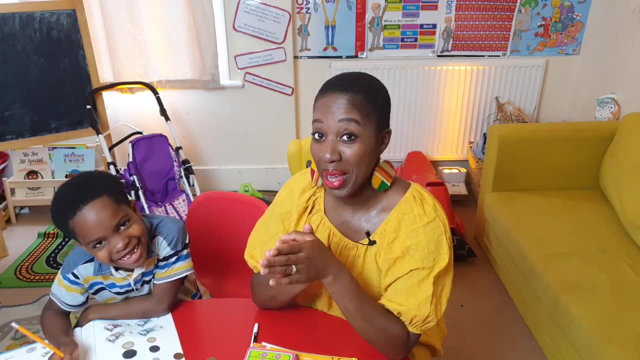 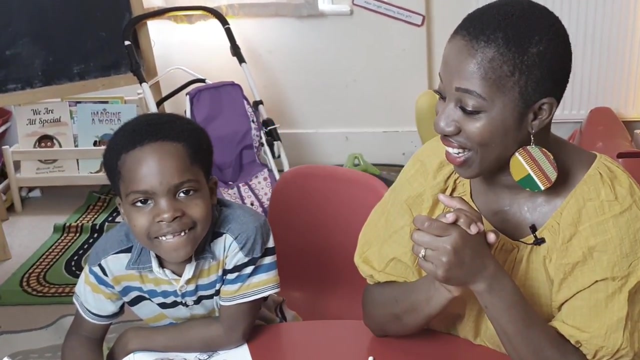 Hello everyone, my name is Zephia Bayayi and welcome back to the Team Bayayi YouTube channel. I'm joined today by our eldest. I'll allow him to introduce himself: Benjamin Rai, Katachia Bayayi. Okay, great, So this is our eldest. I call him Katachia, which is his Ghanaian name. 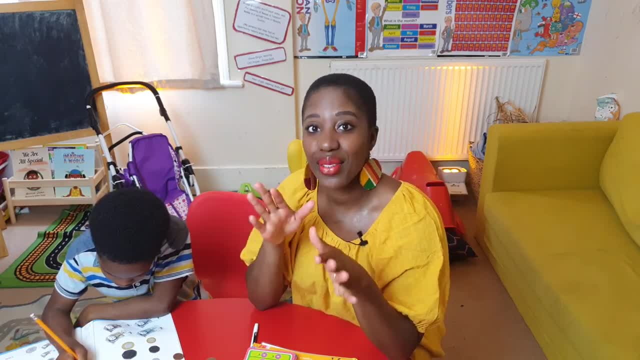 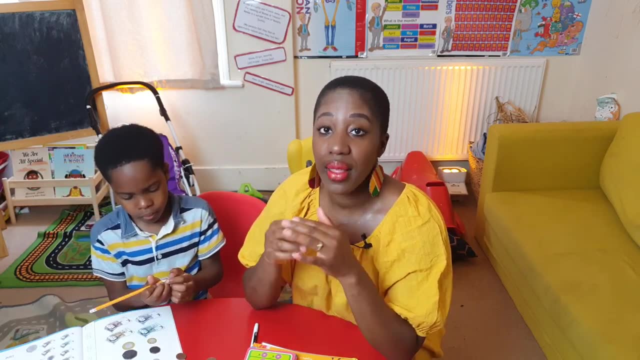 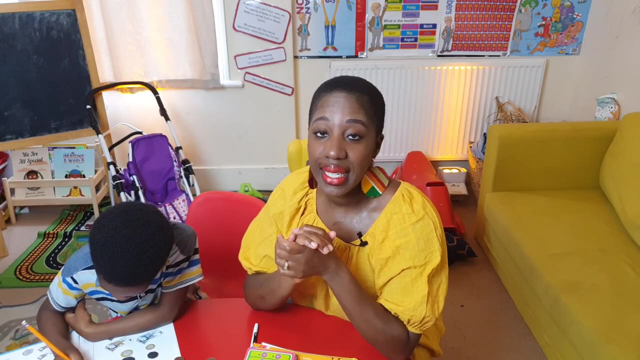 And he's been looking forward to this. He's seen the videos from his brother and sisters. So what we're going to do today is we're going to be talking about how to teach your children the times tables. When I was growing up, maths was an issue subject for me. It wasn't a subject that I was very confident in. 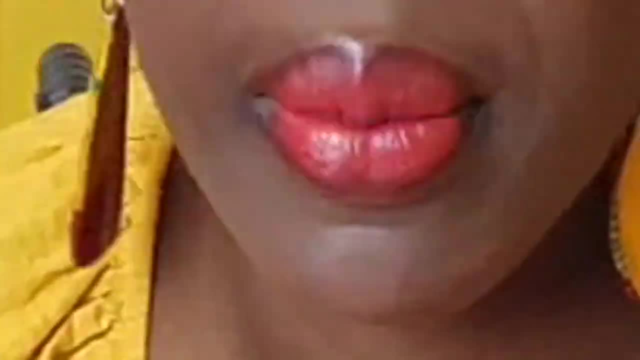 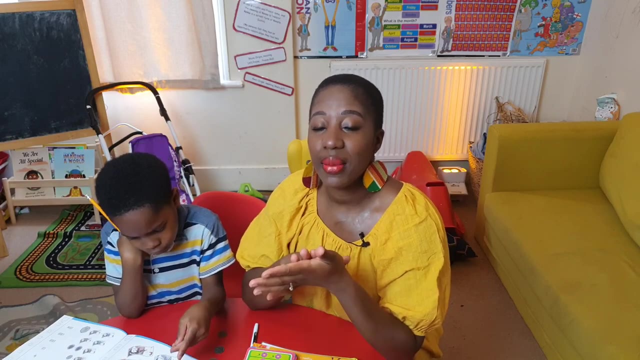 As you become a parent, that narrative stays: I'm not good at maths, I'm not good at maths, And if you keep on kind of speaking life into that, it can easily pass on to your children. So it's something that I deliberately do. 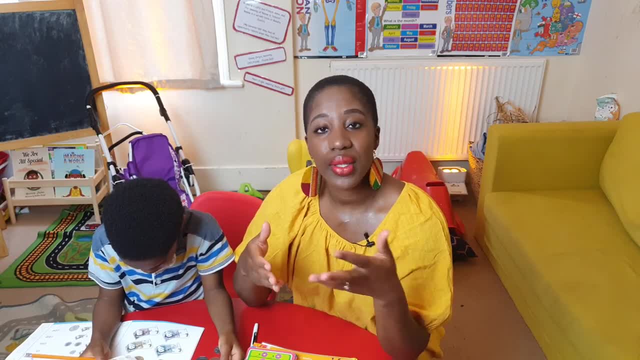 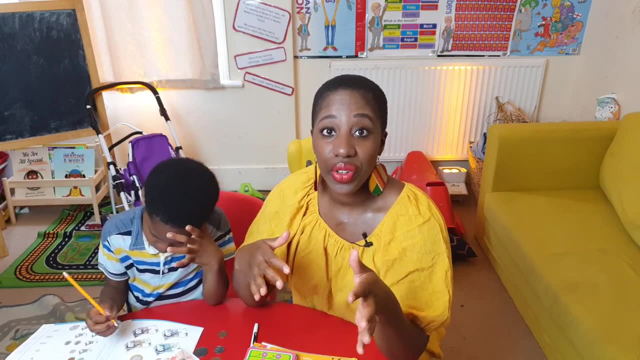 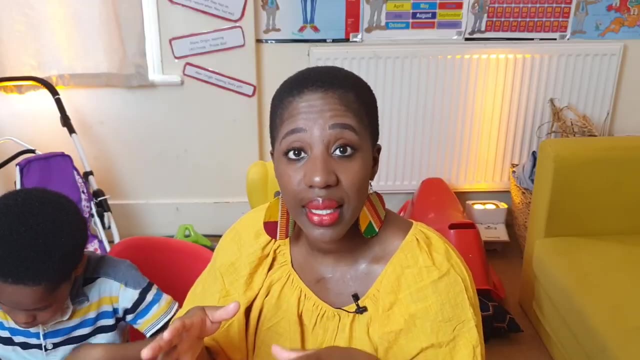 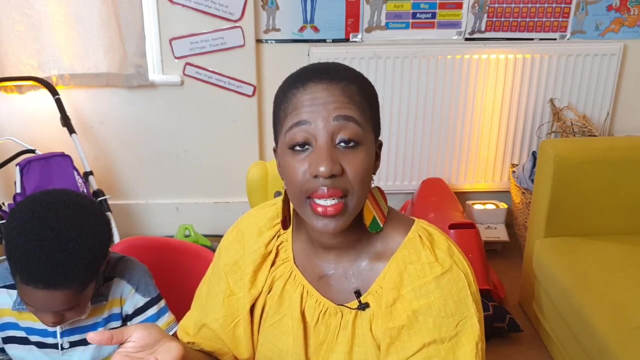 Don't say, because sometimes parents feel that because they're not an expert or they're not brilliant at a particular subject or topic, they're not equipped to teach their children. However, that's not the case. When I was teaching at secondary school, many, many times I would have to sit with the material prior to the lesson and go over it and teach myself before I was then confident to deliver it in a class. 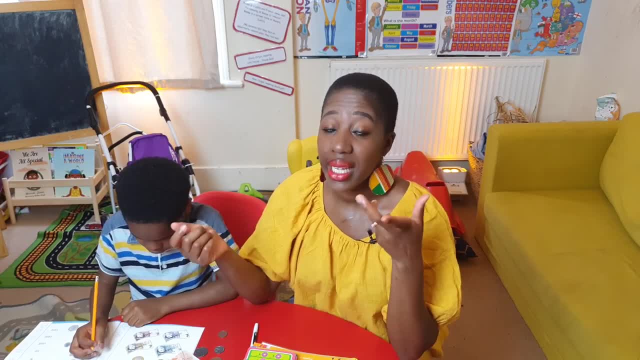 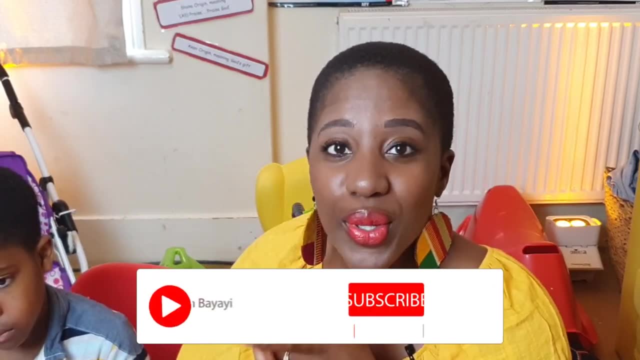 So it's perfectly fine to learn along with your children. It's fun And enjoyable too. Before I continue, I just want to say: don't forget to like, subscribe and also share, and do hit the notification bell so that you are aware whenever we do release videos. 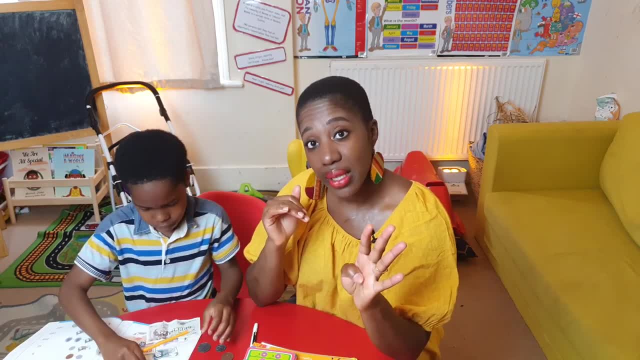 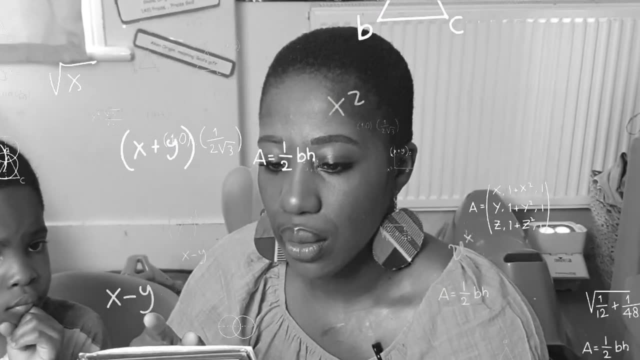 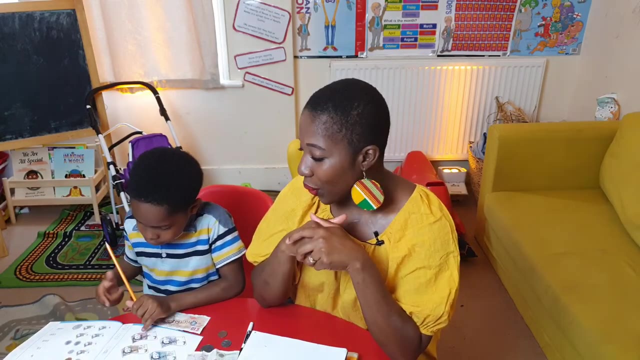 I'm going to look at four approaches to teaching the times tables. Am I? Is it four One? I'm going to be giving you five approaches to teaching the times tables. So, Katya is, how old are you? Seven, Seven years old. 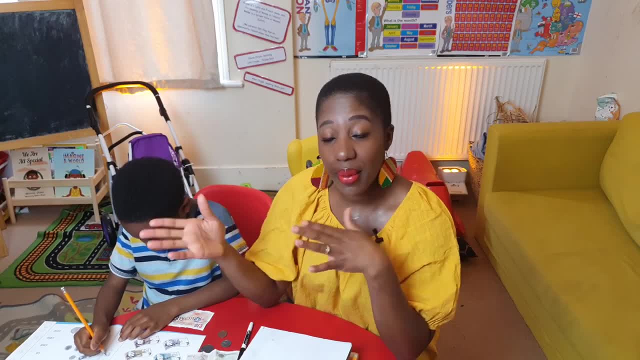 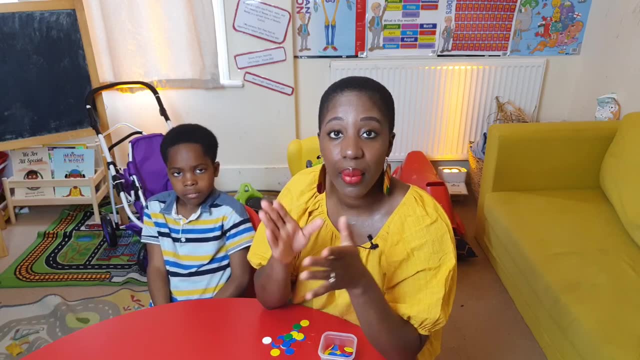 Okay, And what we're going to do is we're going to be demonstrating. you know some of the techniques that we've been using with him. So the first technique or the first approach, is that times tables is a type of repeated addition. 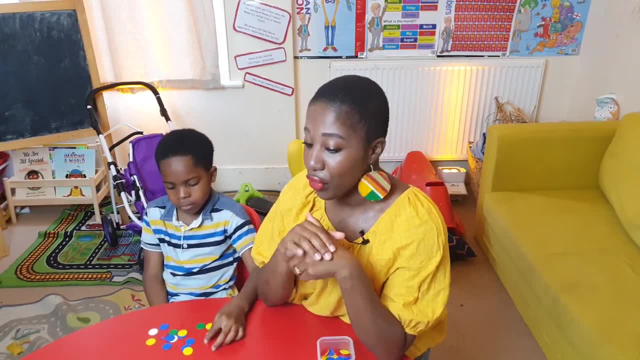 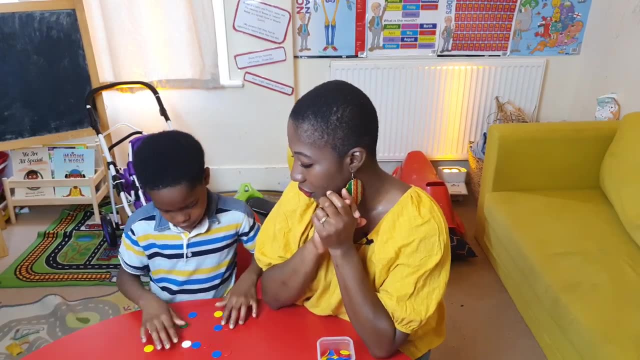 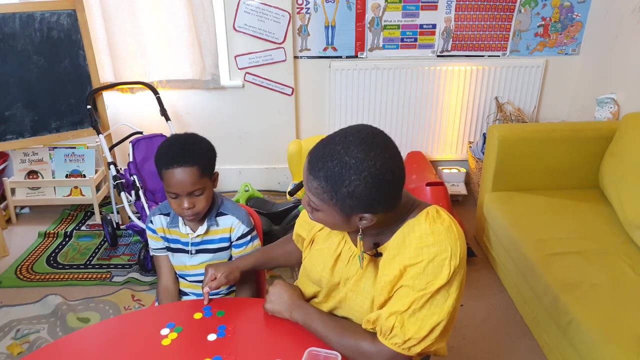 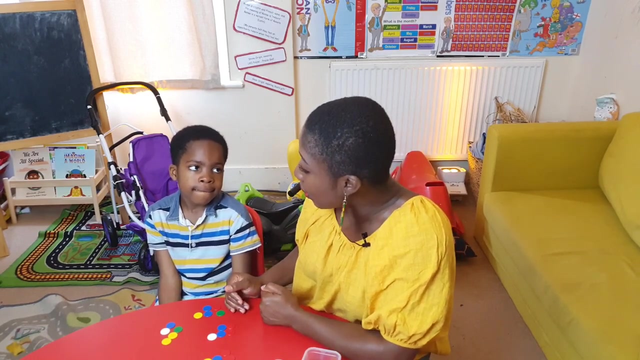 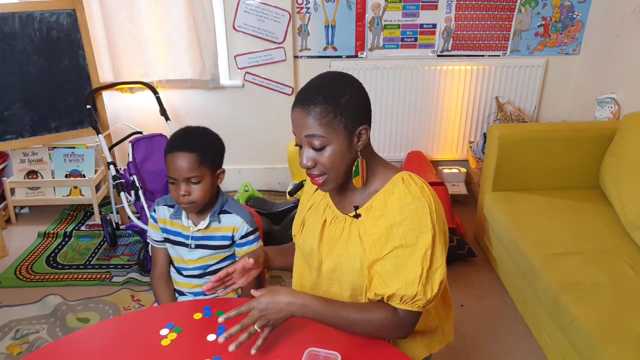 So have a look over here: Four times five, I want four groups of five. Four groups of five is the same as four times exactly, And the answer is twenty. Okay, We're teaching that times tables is a type of repeated addition. 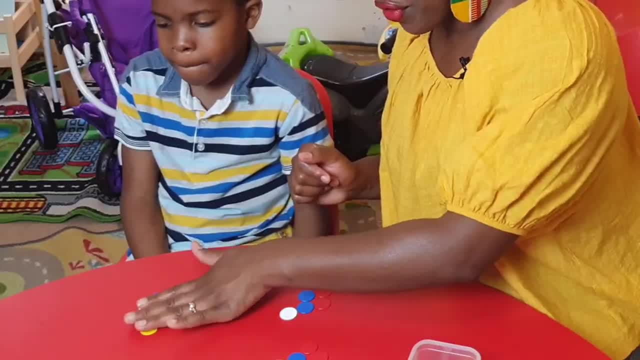 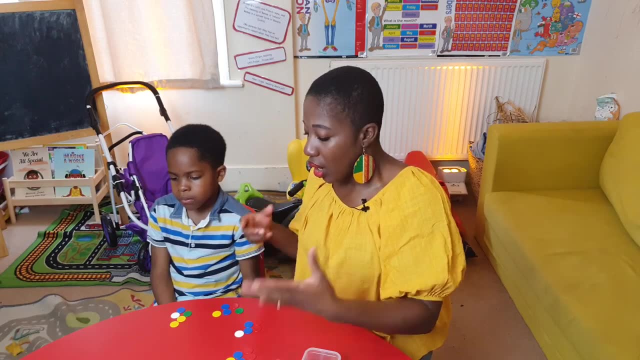 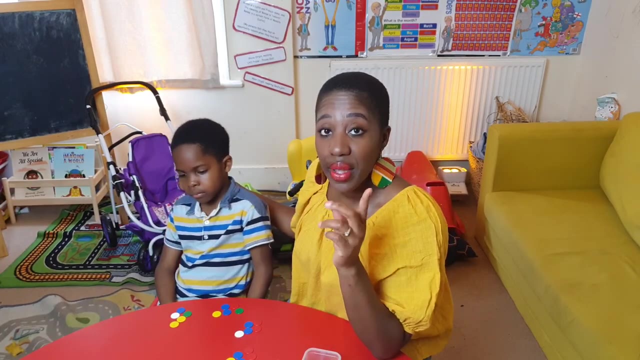 You have five, five, five, five, four times, And in doing that you're using concrete materials. You can use counters, cubes, pasta, but that really helps. And Kids TV 123 have some videos and I'm going to provide the links for that. 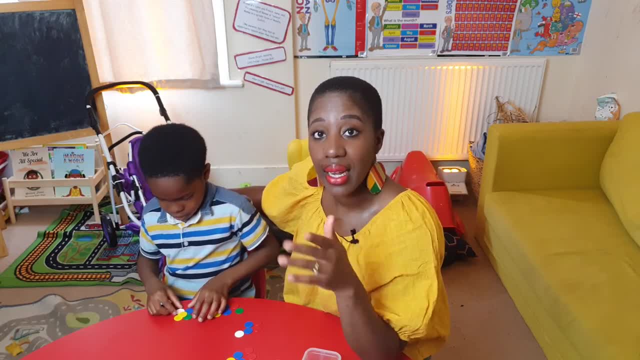 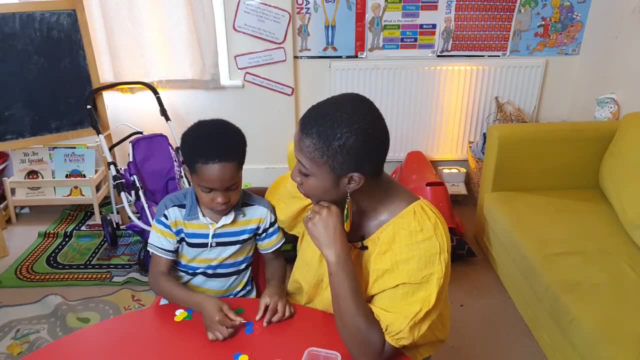 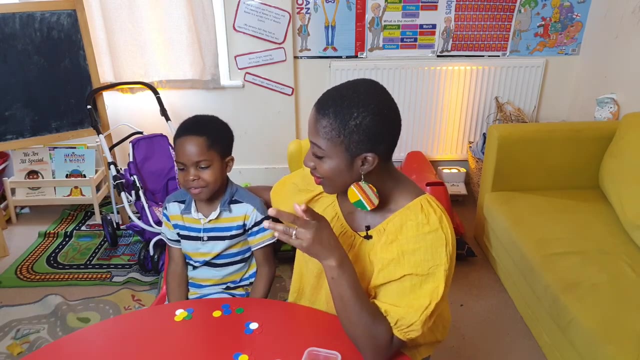 And their tunes are brilliant. Just having that on repeat and learning those songs really helped teach the children how to count in five. So can you count in fives for me? Five, ten, fifteen, twenty, twenty-five, thirty, thirty-five, forty, thirty-five, thirty, thirty. 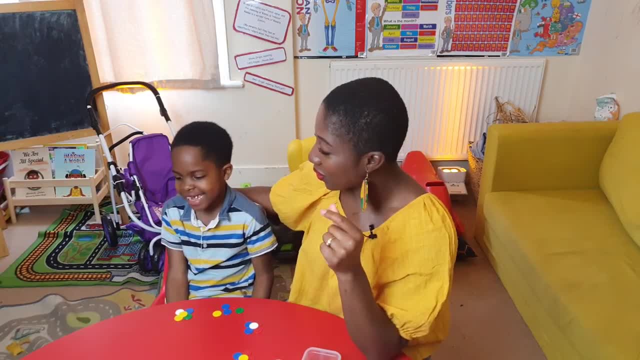 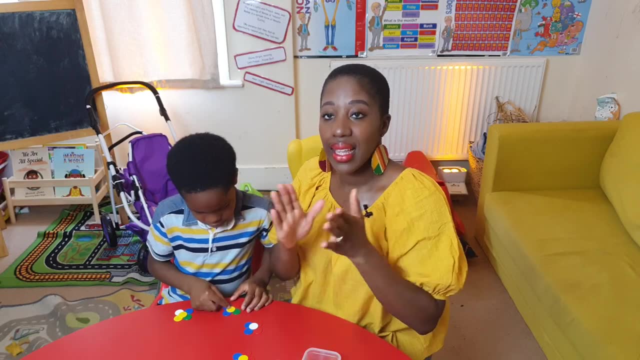 Fifty-five, sixty, fifty-five, seventy, seventy-five, fifty, eighty-five, ninety, eighty-five, ninety and a five. One hundred and one hundred. Yeah, that's how the song goes. That's the second technique in terms of teaching how to count in. you know twos, fives and tens. 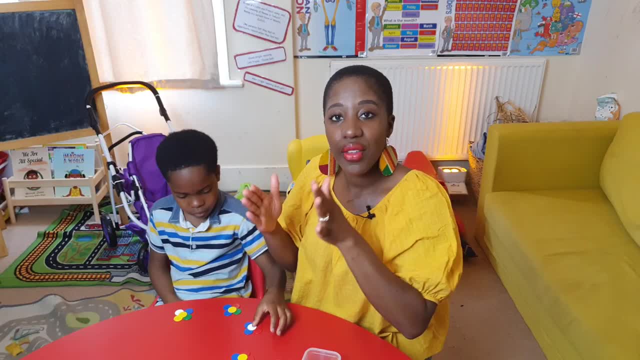 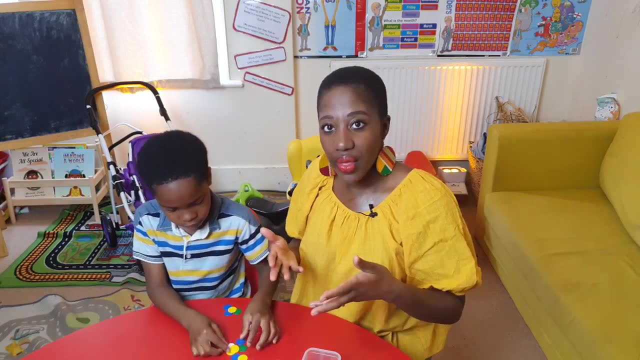 And when it comes to times tables, we always start with the twos, the fives and the tens, because they're a lot more straightforward. So it then gives them a lot more confidence. and then you approach the other times tables. The third technique. 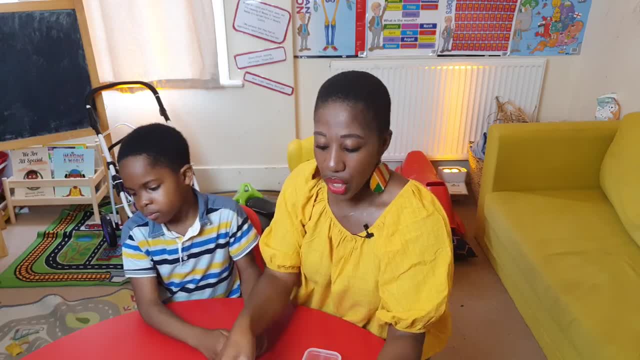 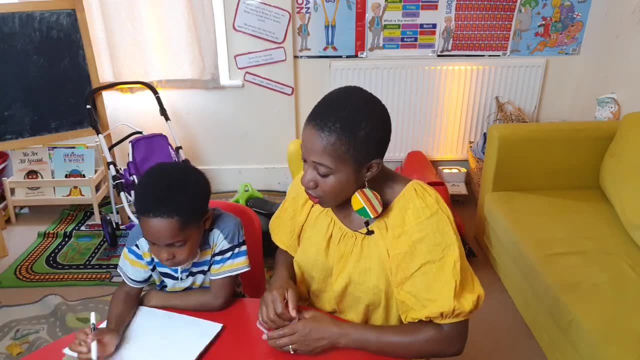 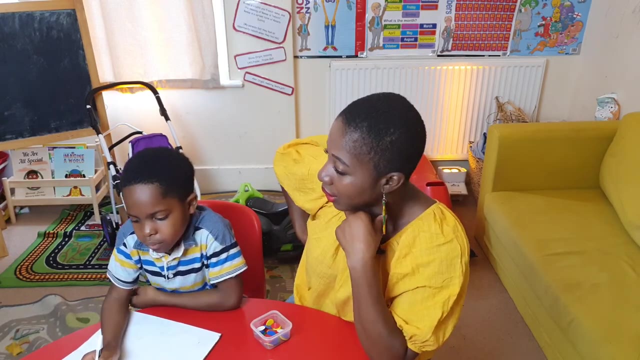 It's teaching them that the opposite is also true. So, Mr Bayayi, could you please write two times nine? So what's the opposite of two times nine, Nine times two? Okay, so write that underneath Right. so what's the answer? 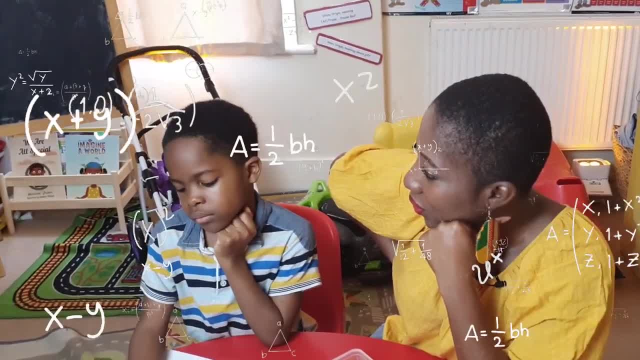 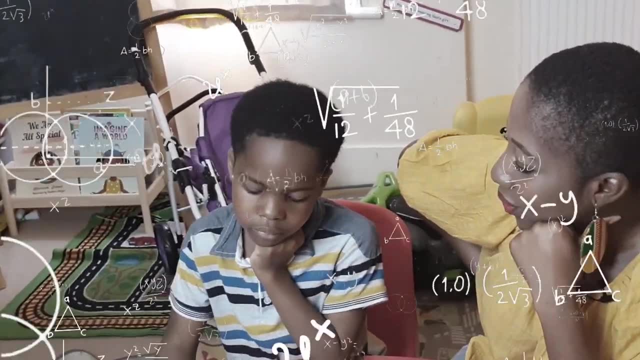 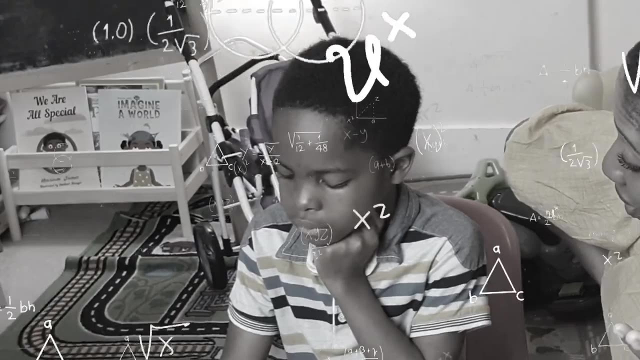 Hello, darkness, my old friend, I've come to talk with you again Because a vision, softly Creeping, Left its seeds while I was sleeping. What's the answer? Tell them so that we can hear: Eighteen, Eighteen. 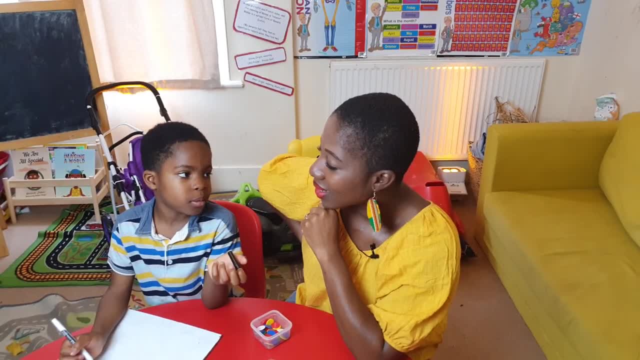 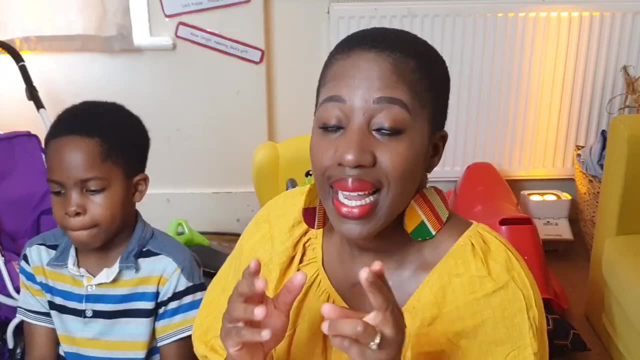 Did you go through your two times tables or your nine times tables? Two times tables? You went through that in your head, okay, And so it's teaching them that the reverse is also true. So that's number three. Now technique. number four is actually drilling. 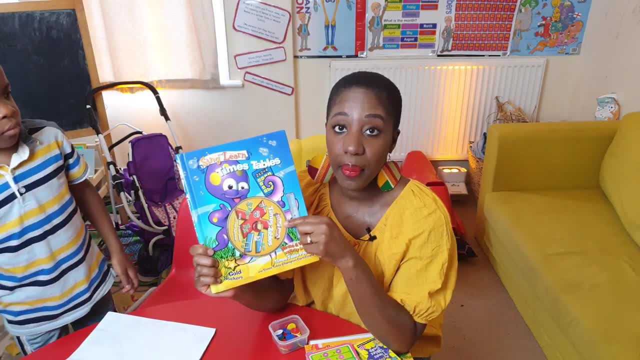 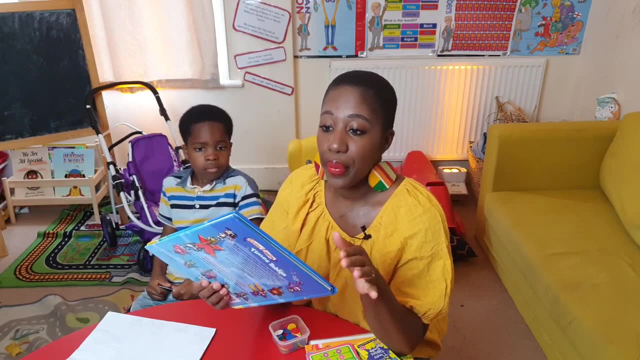 The song that we're about to play is from this book, which I am briefly introducing. I introduced to you in our last video with bar four And that was to do with telling the time, but I touched on the times tables in that. 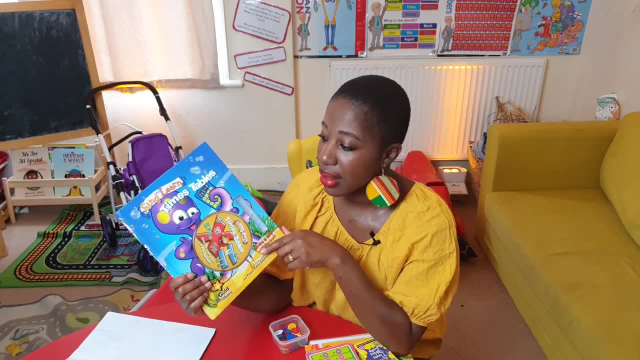 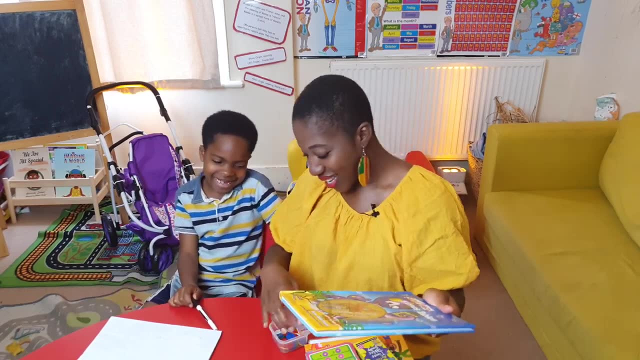 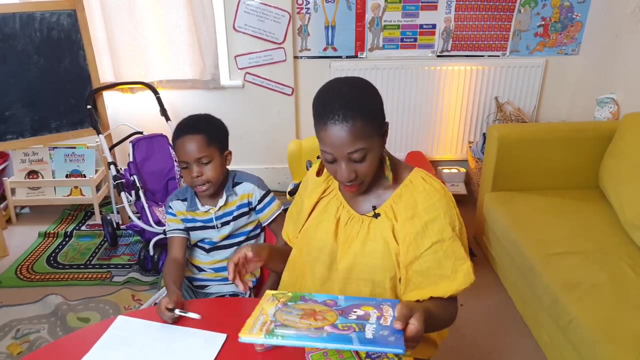 You can purchase this from Amazon. I'm going to provide the link for this. One, two, three, four. Move your shoulders. Come on, All right now. Oh yeah, Six to the fourth, Seven to the fourth, Eight to the sixth. 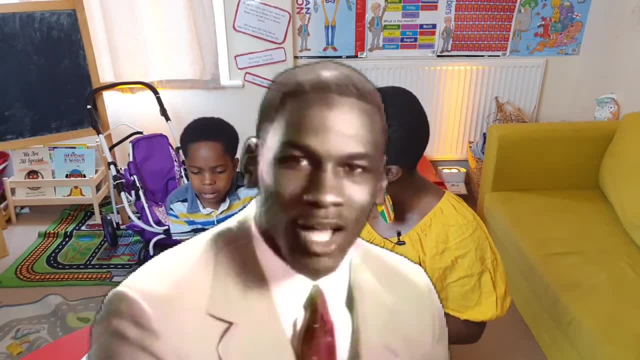 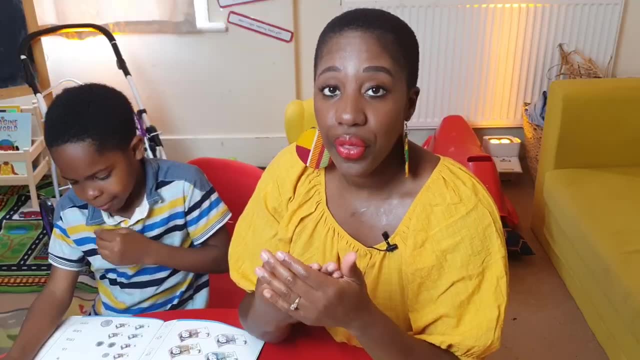 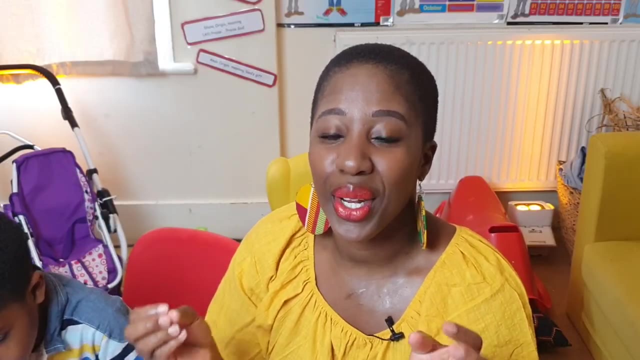 Nine to the eight, Ten to Stop it. Get some help. Okay, so that's the next technique: drilling. So it's literally just going through the times tables over and, over, and over again. Now there's no better way to do that than through song. 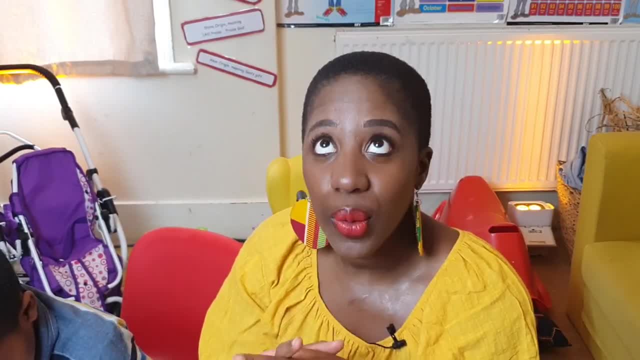 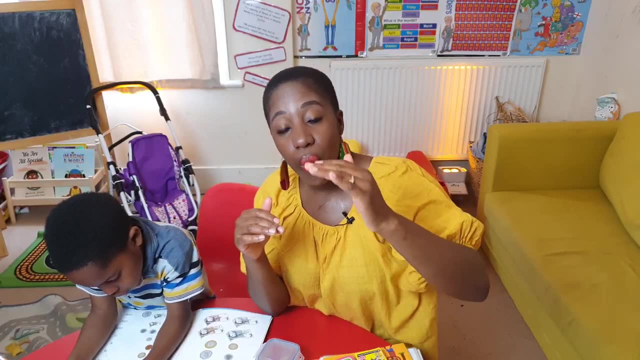 because it helps to commit it to memory and it helps them to recall the information a lot better. You want them to get to a stage whereby they don't have to go through all the times table to get to a particular one. You want them to be able to just answer six times nine. 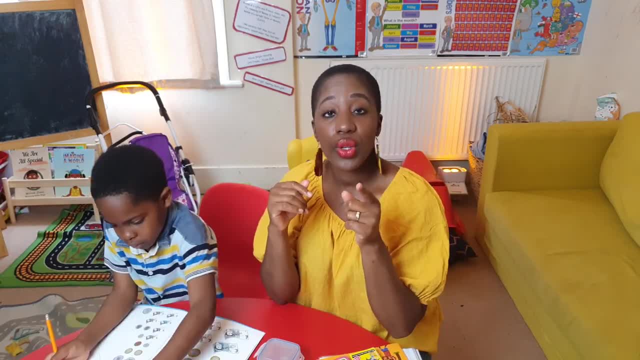 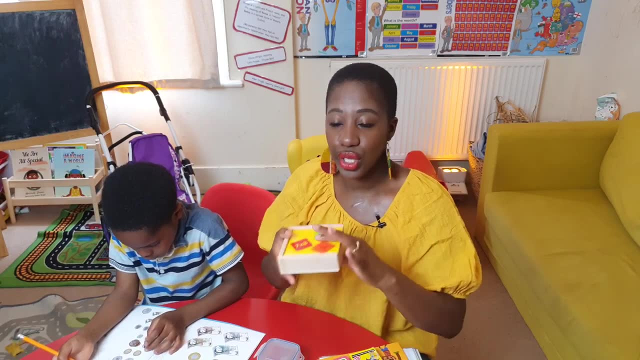 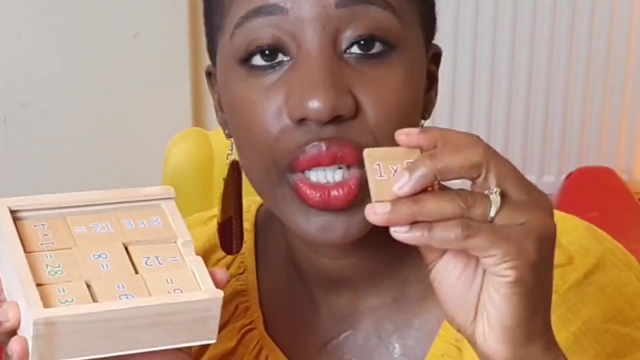 you know, or five times four off the bat. The way in which you do that is through quick fire questions. We actually have this, which I purchased from Aldi, and it is the times tables in, you know, on wooden cubes. It has the answers on the back. 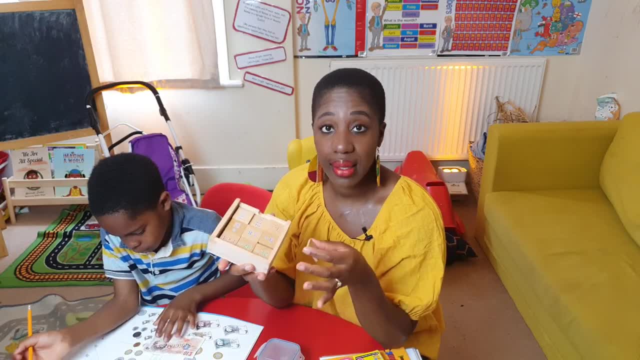 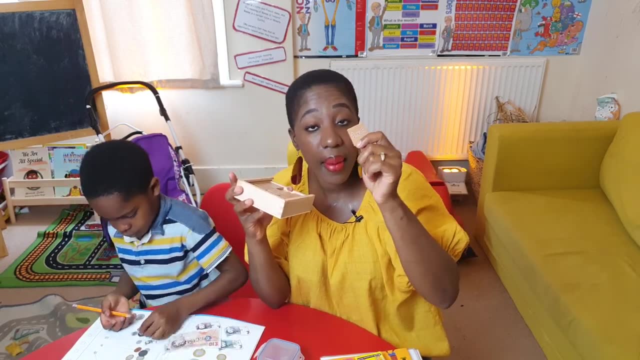 And so before every lesson we usually play a game in relation to that subject, And this is one of the games We do. so are literally just give them random sums and they have to try it and then figure out the answers and they turn it around and they're like: 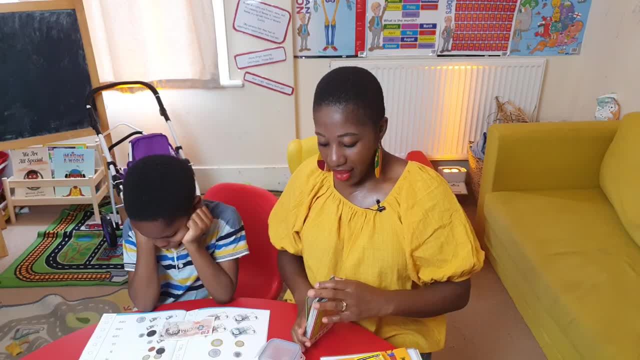 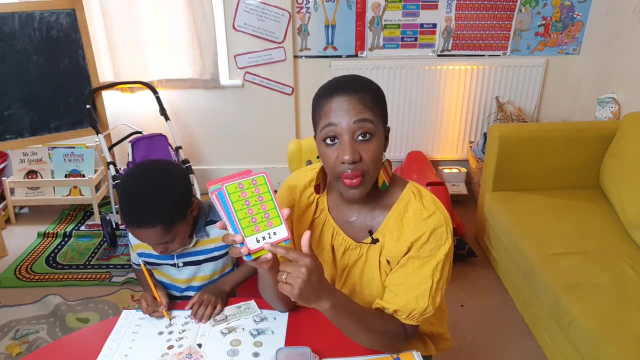 oh, is the right answer is the right answer. and then it has the answer on the back. This: I either purchased it from Aldi or from Lidl, or from Lidl, I can't remember. So this is essentially the same thing. You have the sum on the front and then you have the answers on the back. 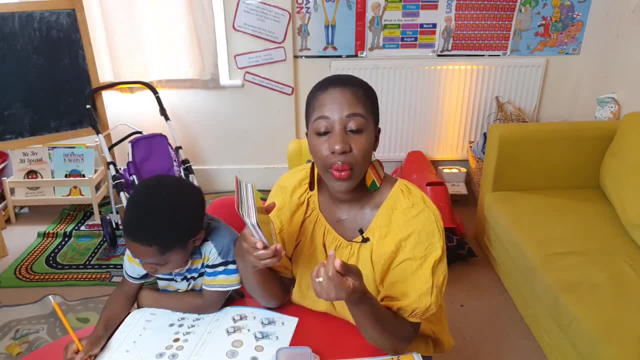 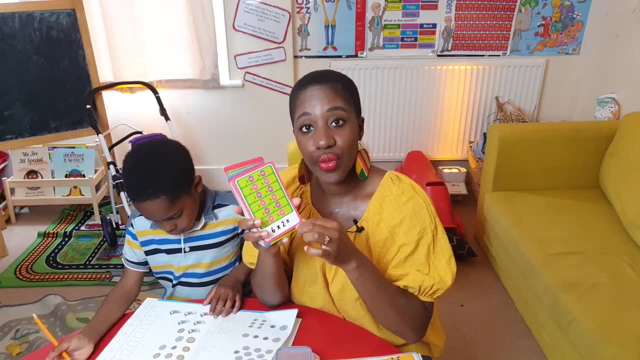 You know you do quick fire questions with them. They're going to get to a point whereby they don't have to keep going through the entire times tables in order to recall what the answer is. If you are able to purchase something like this. 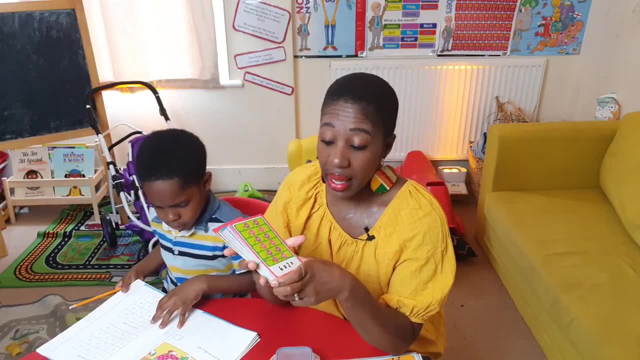 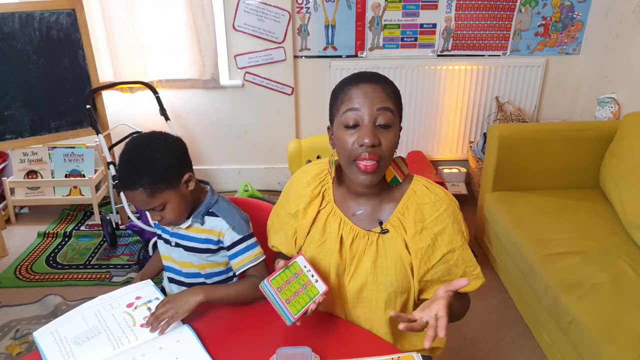 you can just always make it yourself, create the cards and then you can laminate them so that they're durable and they're easy and they last longer. Then you can even, like, set a timer to it, and they've got to try and beat the clock, for example. 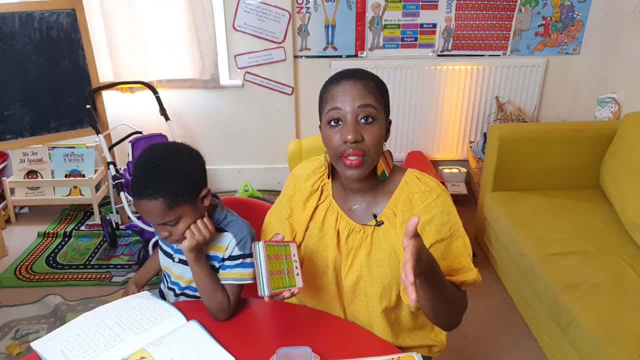 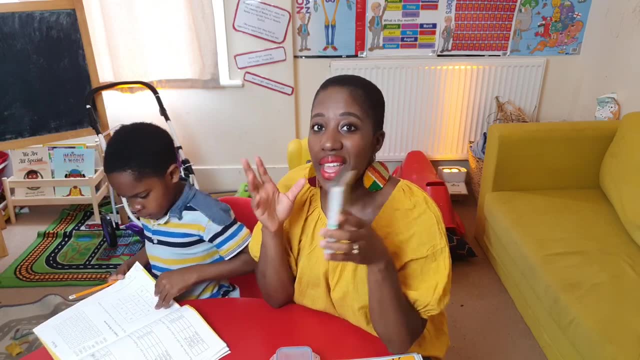 or perhaps they've got to do a certain amount within a particular period of time. So you can make it fun, and when children are having fun they learn a lot better and it doesn't feel like you know they're studying. Going back to the point of drilling, 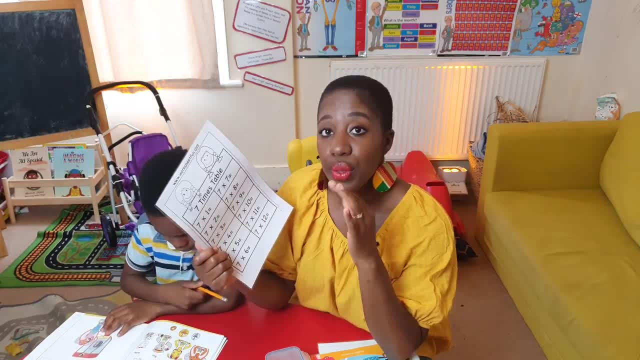 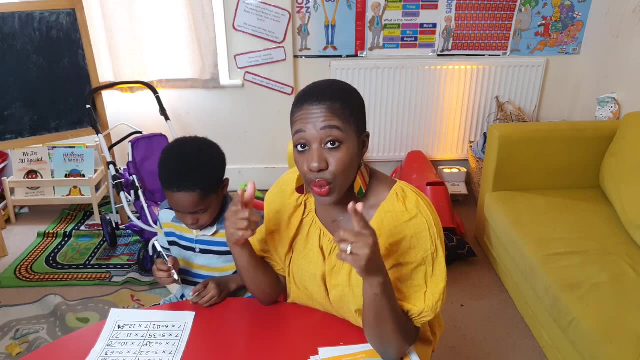 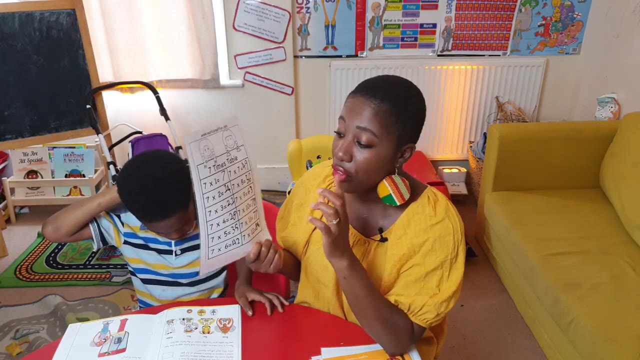 One of the things that I do recommend is, as they are listening to the CD, they would actually go through and write the times tables. that it helps you to process the information better and it helps you to remember the information better. I'm going to provide the link for these sheets that all of the times tables worksheets. 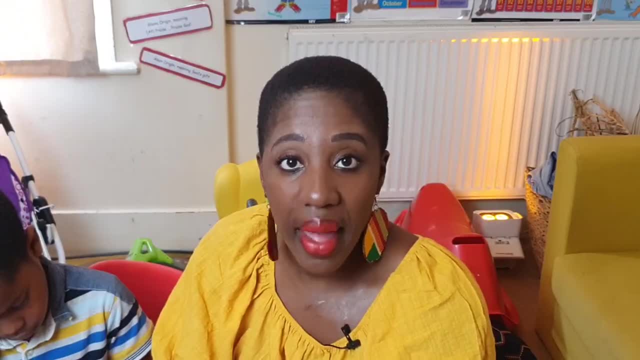 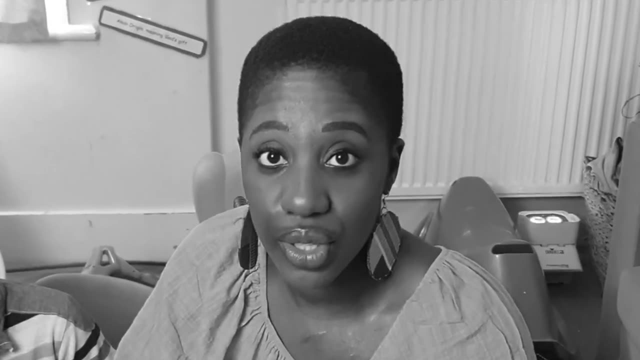 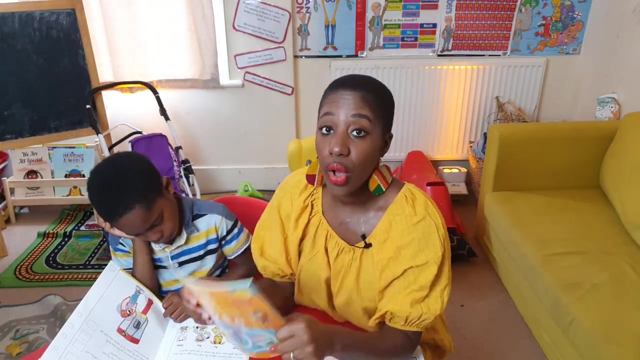 The last point that I wanted to make is teaching them- And I can't actually remember now like how many approaches or techniques have. I've lost track- But the last thing I wanted to mention was teaching them that multiplication is the opposite of division. 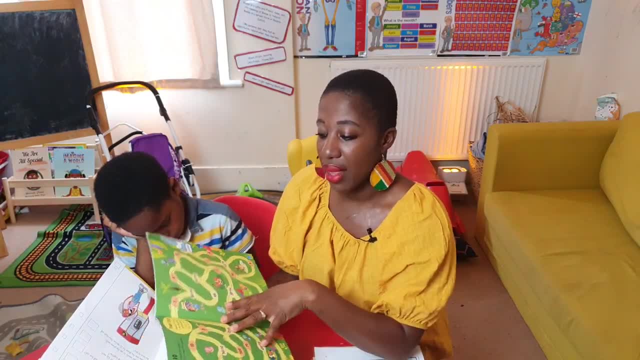 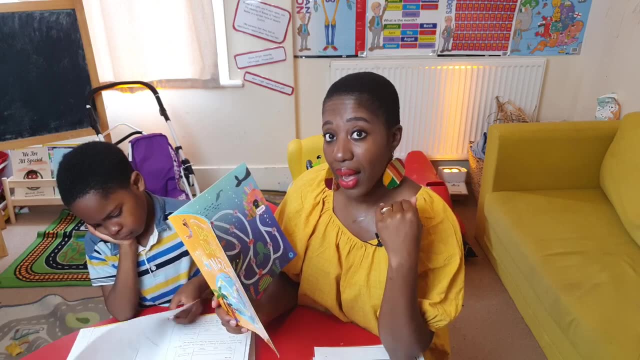 And we are actually, you know, working through this book at the moment, which I purchased from Poundland. It's all about division. in order for him to work out the answers, I just say to him: Okay, Well, do you remember what the opposite is? 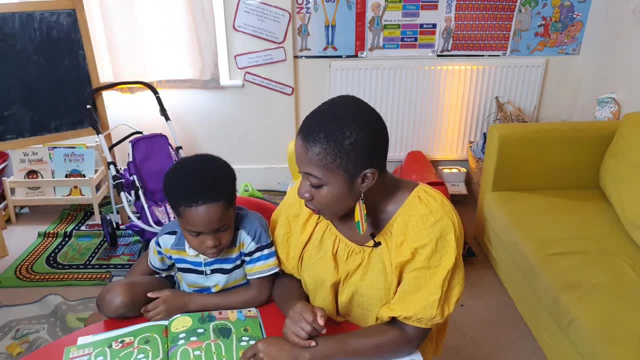 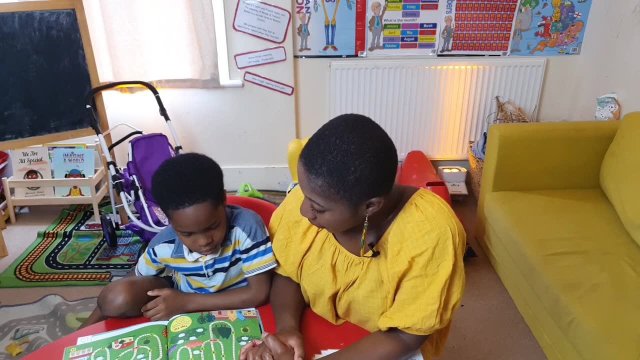 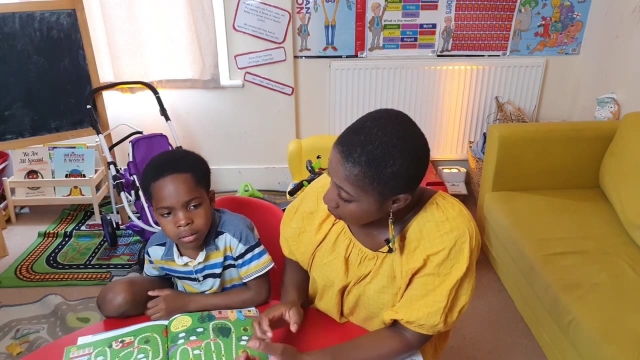 In terms of the opposite being true. So what did you afford? 36 divided by 4 is what 9.. And how did you work that out? My four times tables. So four times what 9.. Is what 36.. 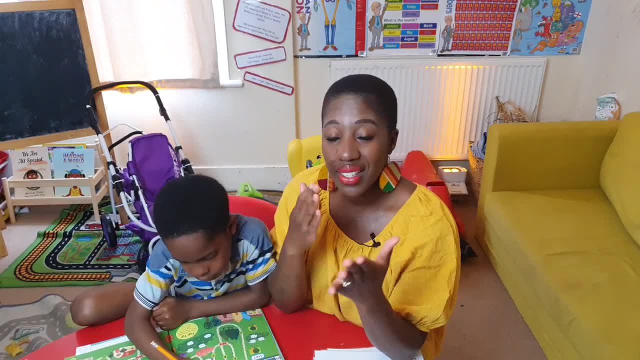 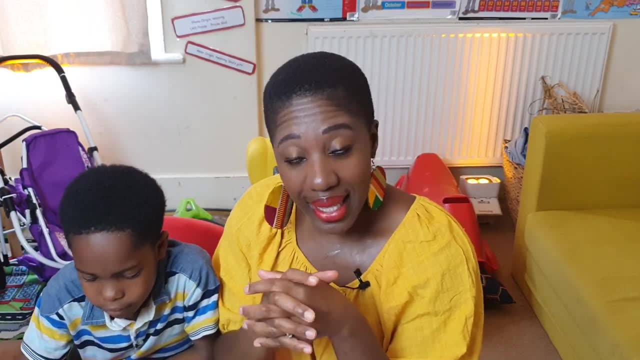 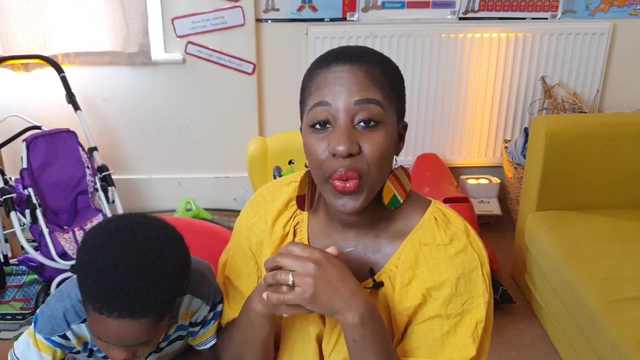 Yeah, Okay, So it's teach them that the opposite is true, That division is the opposite of multiplication, And it's just another angle, It's another approach, It's another technique. That's been it for today's session. Those are the techniques and approaches that I wanted to go over with you, that I feel that I'm will.